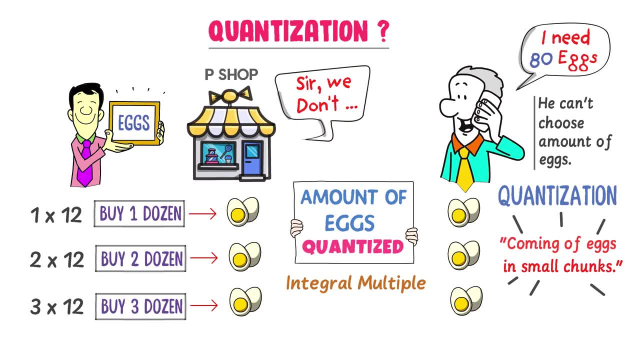 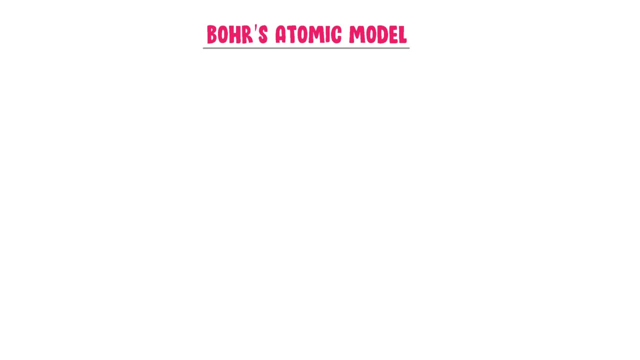 professor noted down that quantization means something coming in small chunks or in small packets which have fixed value or integral multiples. Now let me teach you the main points or postulates of Bohr's atomic model. He stated that electrons revolve around the nucleus in fixed circular paths called orbits or shells, having definite. 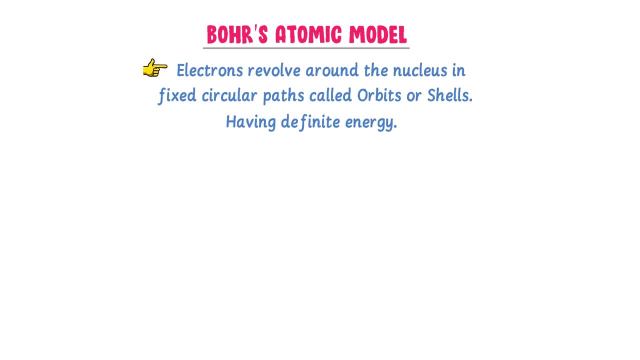 amount of energy or quantized energy. For example, when n is equal to one, it is k-shell, When n is equal to two, it is l-shell, When n is equal to three it is m-shell, And when n is equal to four it is n-shell. 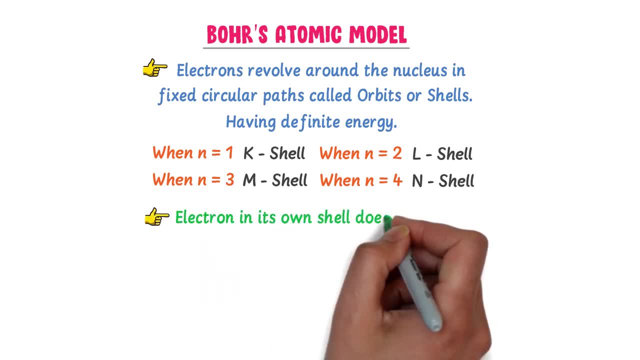 Secondly, he stated that electron and its own shell does not lose Argan energy. It loses Argan's energy when it jumps from one shell to another. Thirdly, he stated that electrons revolve around the nucleus in fixed circular paths or into a new path or a new state in. 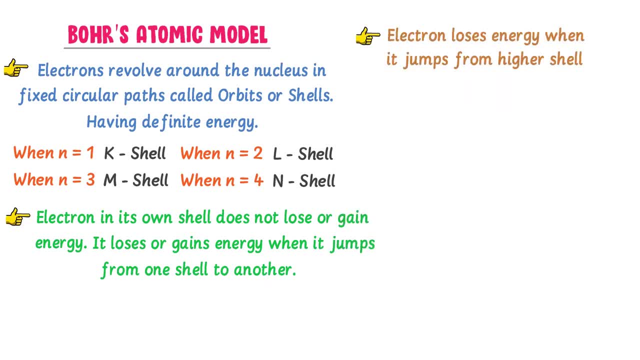 that electron loses energy when it jumps from higher to lower shell, while it gains energy when it jumps from lower to higher shell. Remember that it loses or gains the same amount of energy while jumping from one orbit to another. Fourthly, he stated that the angular 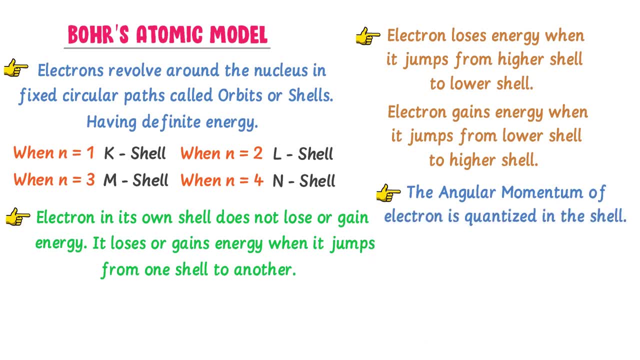 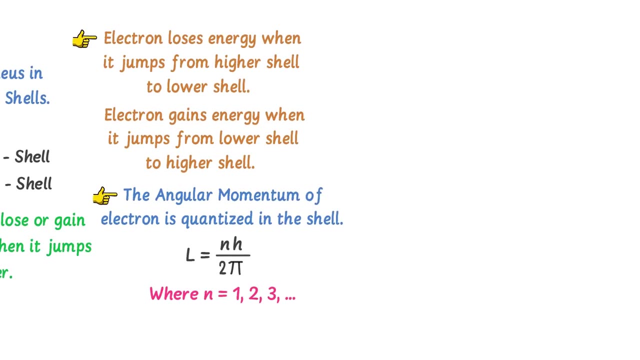 momentum of electron is quantized in the shell, which is: L is equal to nh upon 2π, where n is multiple of natural number and h is Planck's constant. Here let me explain two important points. angular momentum of electron is quantized and integral, multiple of natural. 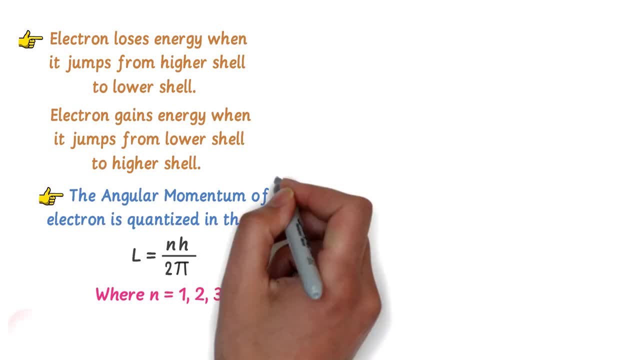 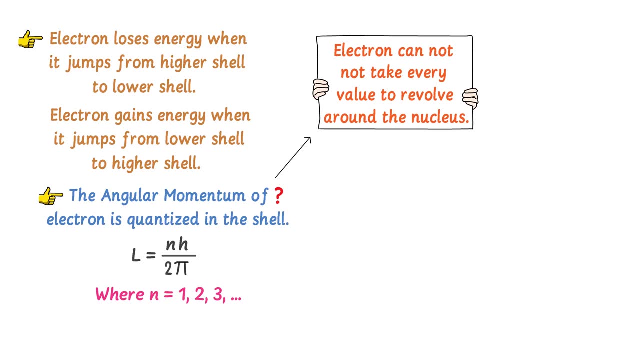 numbers. Well, angular momentum of electron is quantized means that electron cannot take every value to revolve around the nucleus. Electron can take either 1h upon 2π, 2h upon 2π, 3h upon 2π, 3h upon 2π, etc. but electron can take any value to revolve around the nucleus. 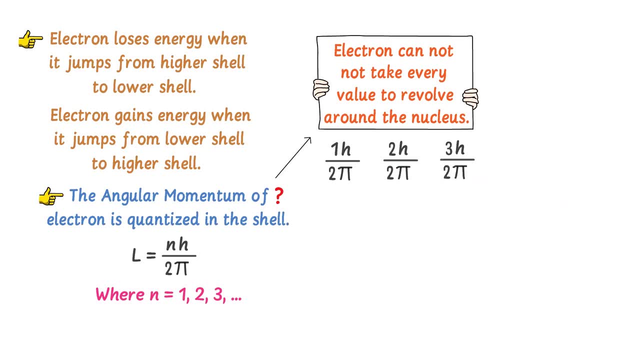 2π, 3h upon 2π are so on values to revolve around the nucleus. Secondly, angular momentum is integral. multiple of natural numbers means that n can take 1,, 2,, 3 and so on values. Also, we know that angular momentum is: L is equal to mvr, where m is the mass of electron. 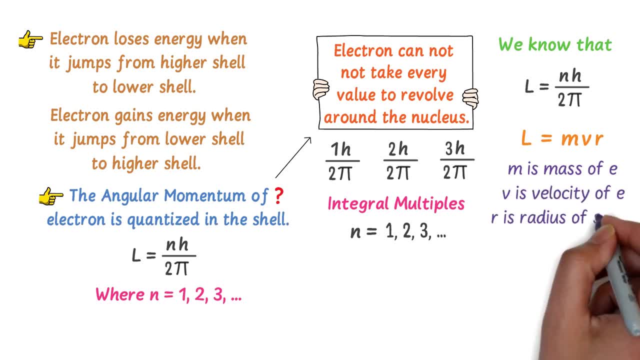 v is the velocity of the electron and r is the radius of the shell. Putting the value of L in this equation, we get mvr is equal to nh upon 2π. Note it down, this equation, because I will play with this equation many times in this. 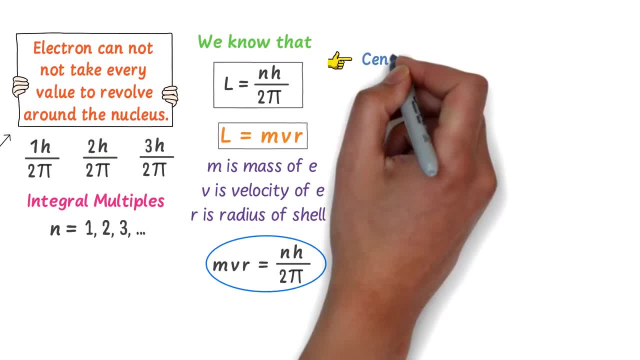 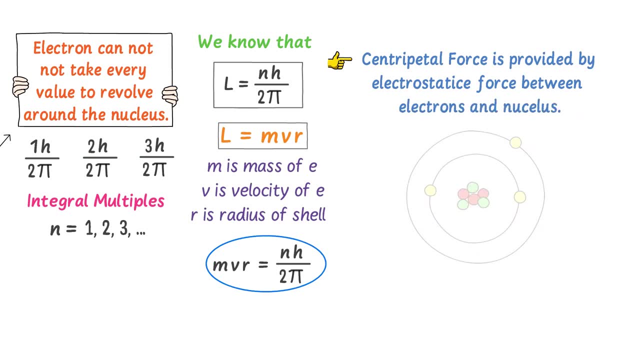 lecture. Fifthly, he stated that the centripetal force is provided by the electrostatic force between electrons and nucleus. It means that electron revolves around the nucleus, so it needs centripetal force, Fc, which is provided by the electrostatic force or attractive force Fe, between electrons and 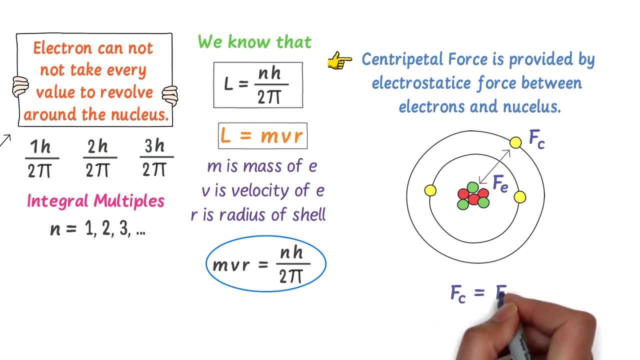 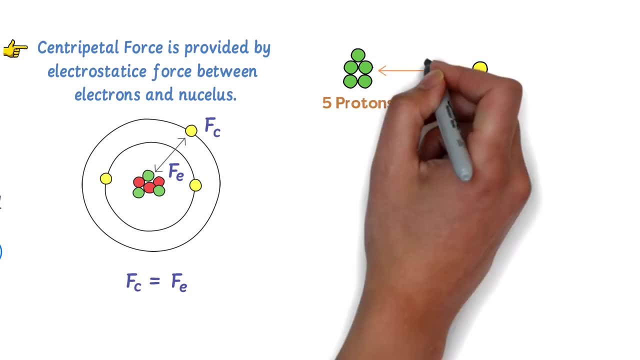 nucleus. Hence we write: Fc is equal to Fe. Now let consider five protons and one electron. Let the distance between them is r. we represent total number of protons by z, which is called atomic number. We know that proton and electron have the same charge, but opposite. 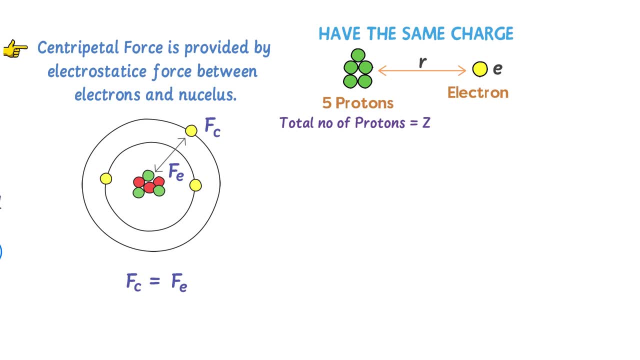 Let. the charge on electron is E. also the charge on proton is E. So there are five protons. I write five proton, or instead of five I write Ze. Now, according to Coulomb-Baba, there is electrostatic force between protons and electrons. 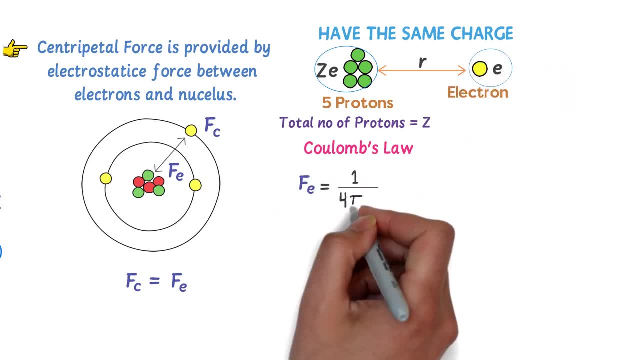 We know that it is Fe is equal to 1.. It is equal to 1 upon 4 pi epsilon and to Ze upon r squared. Also, we know that centripetal force Fc is equal to Me squared upon r. According to Bohr-Baba, Fc is equal to Fe. so I get Me squared upon. r is equal to 1 upon. 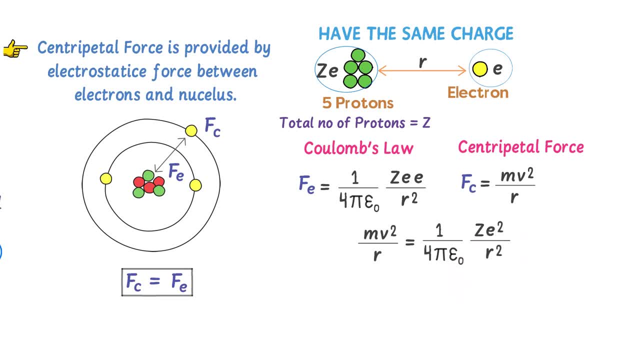 4 pi epsilon, and to Ze squared upon r squared. This r and this r are cancelled. So we know that it is equal to 1 upon 4 pi epsilon, and to Ze squared upon r squared, I get Mv. squared is equal to 1 upon 4 pi epsilon, and to Ze squared upon r. 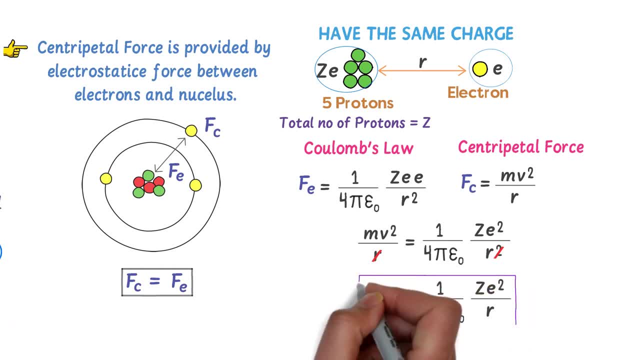 Let- this is equation number two- Also noted down this equation, because I will play with this equation many times in this lecture. Now, on the basis of these postulates, we will derive radius, velocity, kinetic energy, potential energy, total energy of electron and electron. 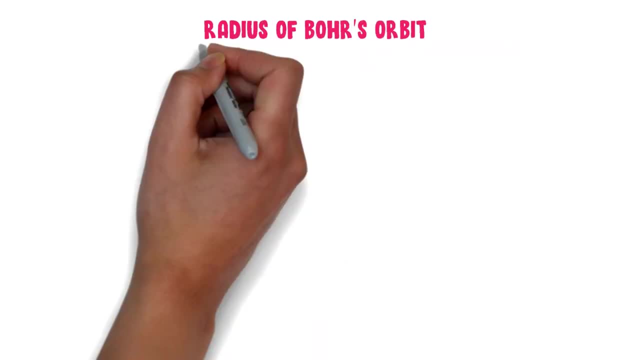 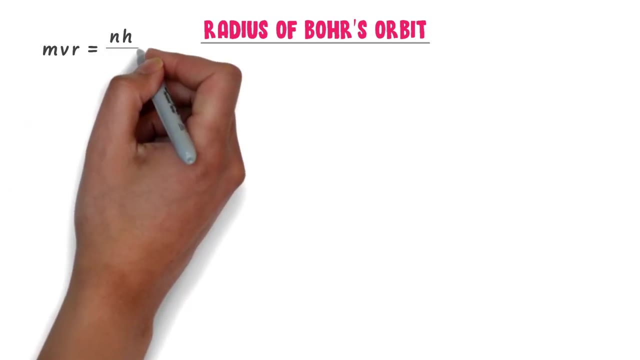 Now let me derive the radius of Bohr's orbit. Firstly, I always write the two equations: Mvr is equal to nh upon 2 pi and mv squared is equal to 1 upon 4 pi, epsilon, and to Ze squared upon r. 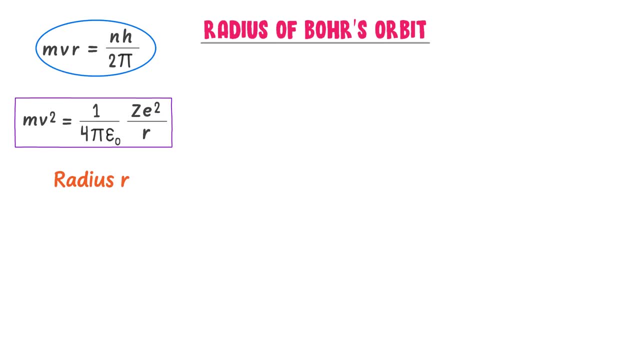 We are deriving radius r of the Bohr's orbit, So r is there in this equation and it is there in this equation. Thus we derive radius r of Bohr's orbit. Now let me derive the radius of Bohr's orbit. 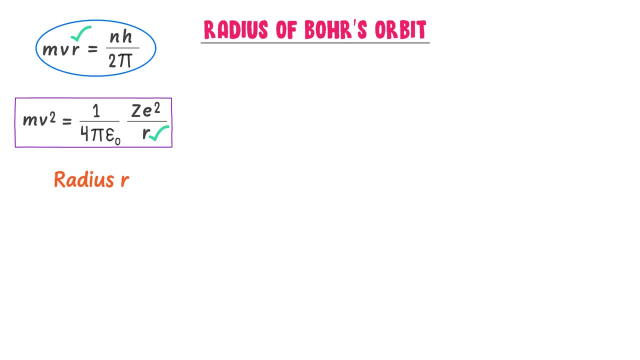 I will use these both equations to derive the equation of radius. Now I take this equation and I write it here. I shift this m from left hand side to right hand side. I get v squared is equal to 1 upon 4 pi. epsilon m into z e squared upon r. 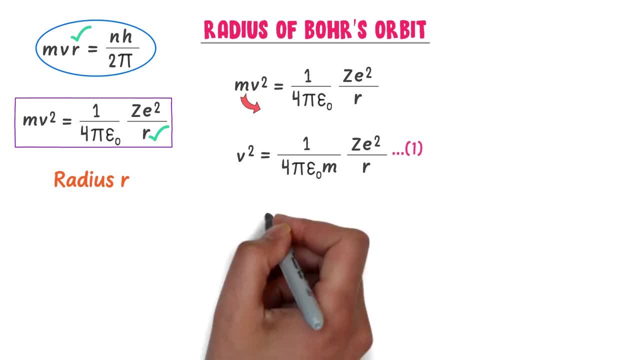 That this is equation number 1.. Secondly, I take this equation and write it here. I square both sides. I get m squared, v squared. r squared is equal to n squared h squared upon 4 pi squared. I shift m squared, v squared, from left hand side to right hand side. 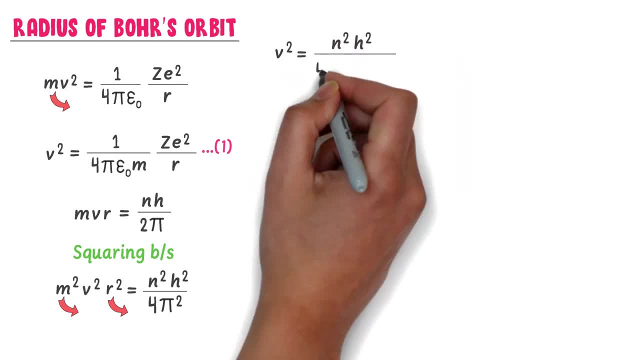 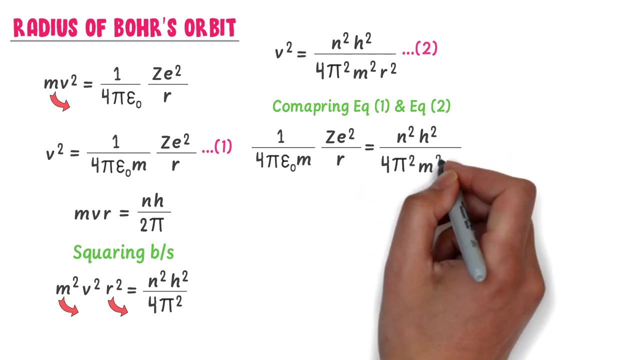 I get: v, squared, is equal to n squared h, squared upon 4 pi squared m squared r squared That this is equation number 2.. Now, comparing equation number 1 and equation 2, we get 1 upon 4 pi epsilon m into z. e squared upon r is equal to n squared h squared upon. 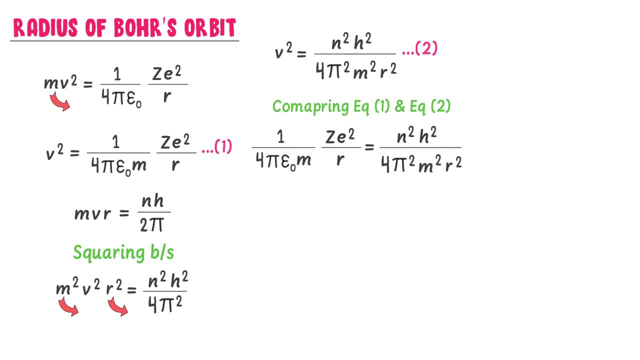 4. pi squared m squared r squared. This 4 and this 4 is canceled. This square of pi is canceled. This m and this square of m is canceled. This r and this square of r is canceled. We get ci squared. 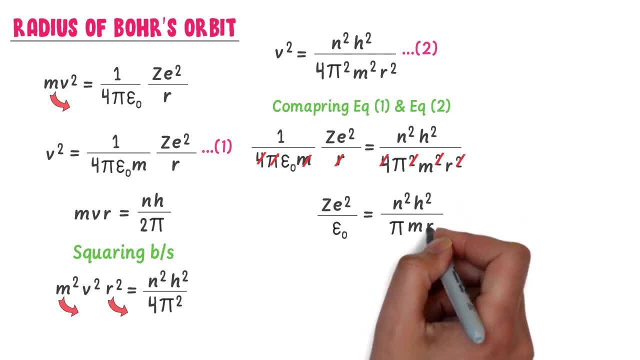 Is equal to 2.. to n square h square upon pi m r, I shift r and epsilon I get r. z e squared is equal to epsilon n square h square upon pi m. Our subject is radius r, So I get r is equal to epsilon n square h. 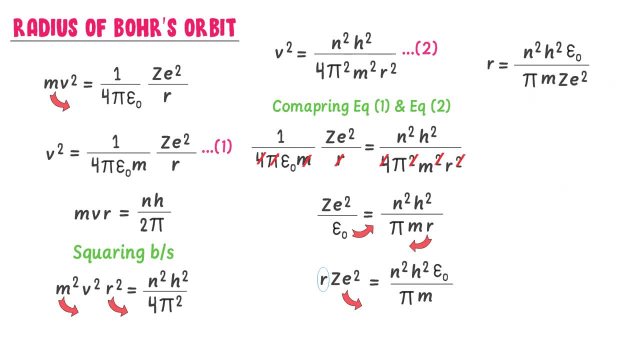 square upon pi, m, z e squared. Now here I separate all the constant terms: r is equal to epsilon, h square upon pi, m. e squared into n square upon z. After putting the values of constants in this equation, I get: r is equal to 0.53, n squared upon z, n strong. So this is the radius of Bohr's. 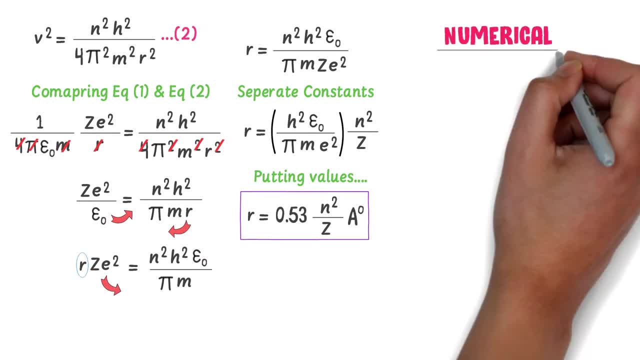 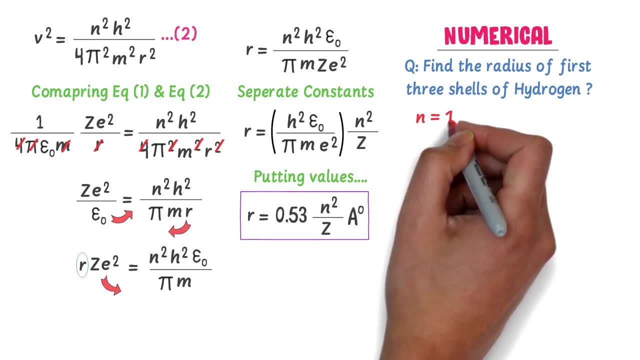 orbit. Here let me teach you one numerical question. Find the radius of first three shells of hydrogen. Well, we know that when n is equal to 1, it is k shell. The atomic number of hydrogen is z is equal to 1.. Also, we derive that r is equal to 0.53, n to n squared upon z, n strong. So we get: 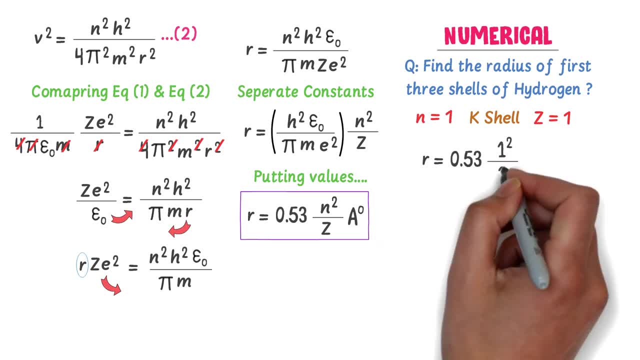 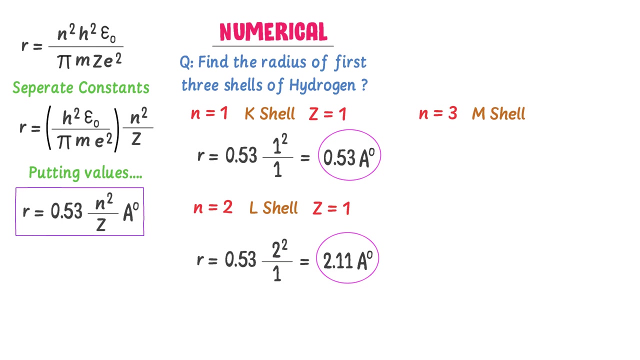 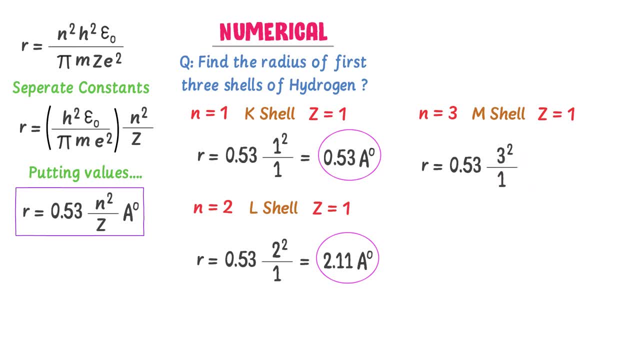 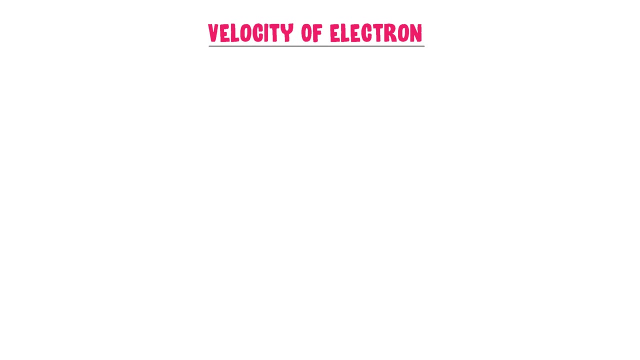 r is equal to 0.53 n to 3 squared upon 1, which is equal to 4.76 n strong. By this way we can calculate the atomic radius of hydrogen. Now let me derive the speed of electron in Bohr's orbit. We know that mv r is equal to n h upon 2 pi. We have already calculated. 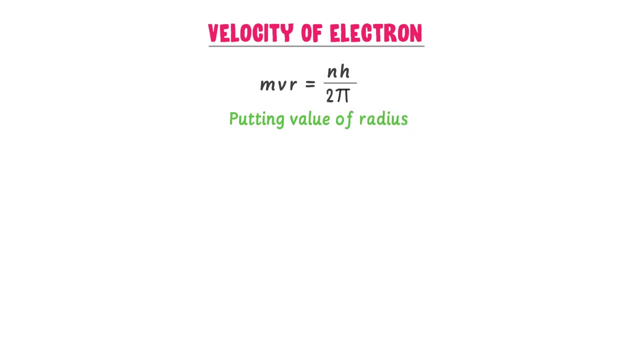 the value of radius. So I will put the value of radius in this equation. I write mv and I put the value of radius. Epsilon. n square, h square upon pi. m. z e squared is equal to n, h upon 2 pi. This m and this m is cancelled. This pi and this pi is cancelled. This n squared. 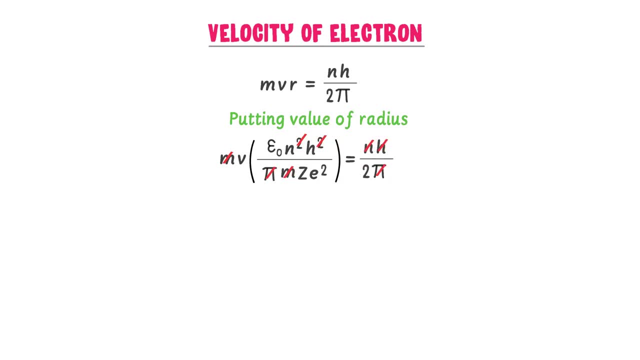 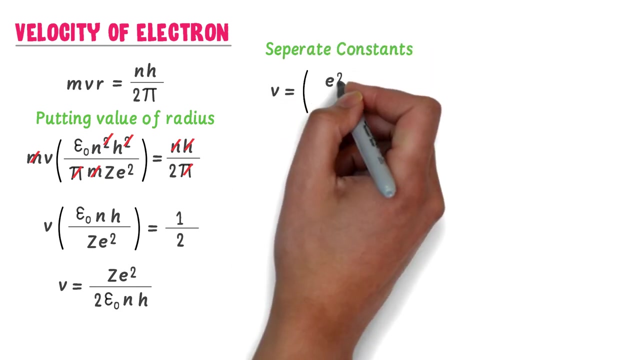 and n is cancelled. This h square and h is cancelled. I get v: n to epsilon n. h upon z. e squared is equal to 1 upon 2.. Rearranging the equation: I get v is equal to z. e squared upon 2, epsilon n- h. I separate the constant terms. I get v is equal to e squared upon. 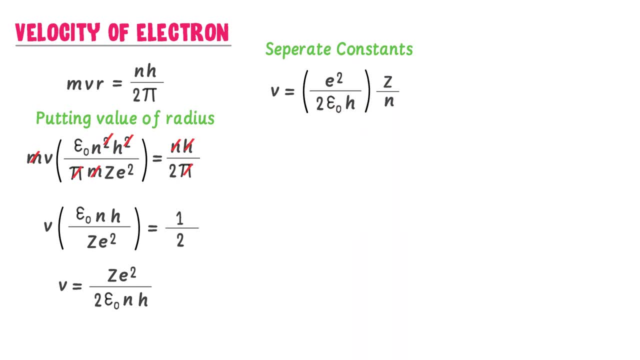 2 epsilon h. n to z upon n. After putting values of constants I get: v is equal to 2.186, n to 10 to the power. 6 n to z upon n m per second. This is the velocity of electron in Bohr's orbit. 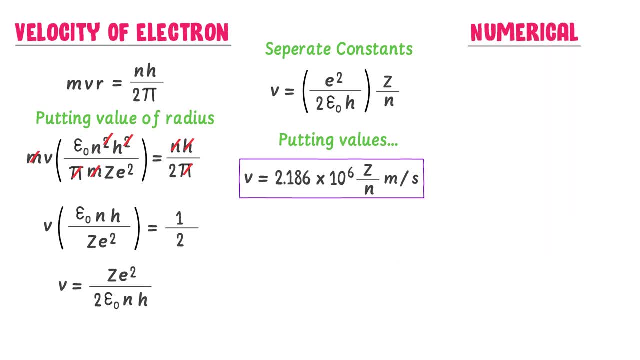 Here. let me teach you one numerical question. Find the speed of electron and second shell of helium. Well, we know that when n is equal to 2, it is second shell. The atomic number of helium is equal to 2.. We also know that the speed of helium is equal to the speed. 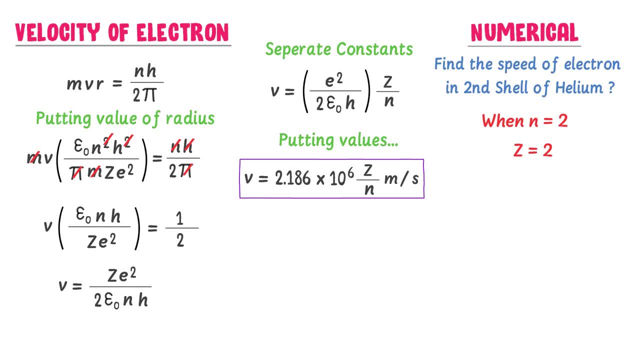 helium is Z is equal to 2.. So we write: V is equal to 2.186 into 10 to the power 6 into 2 upon 2 meter per second. We get 2.186 into 10 to the power, 6 meter per second. So this is the. 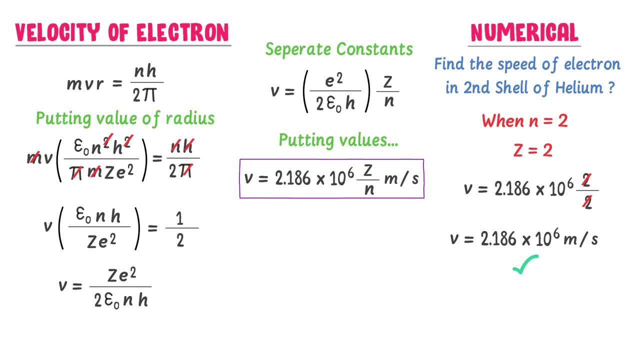 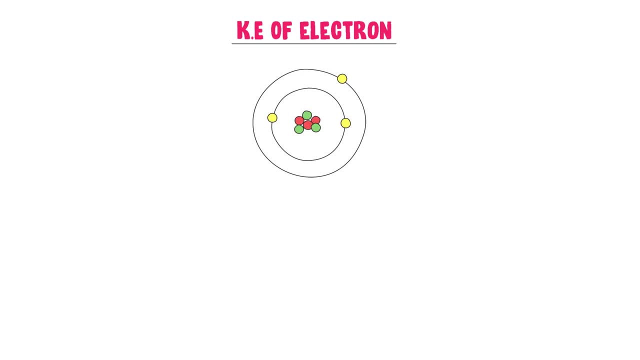 speed of electron and second shell of helium. Now let me derive the kinetic energy of electron in Bohr's orbit. We know that electron is in motion while revolving around the nucleus, So it possesses kinetic energy due to its motion. Also, we know that kinetic energy is equal to. 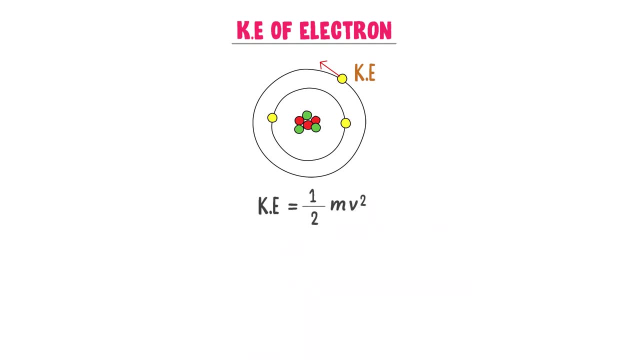 half mv squared. We have already calculated the value of speed of electron. So I write: kinetic energy is equal to half of mass into Ze squared upon 2 epsilon nh. So we get 2.186 into 10, to the power 6, into 2.186, into 10, to the power 6, into 2.186, into. 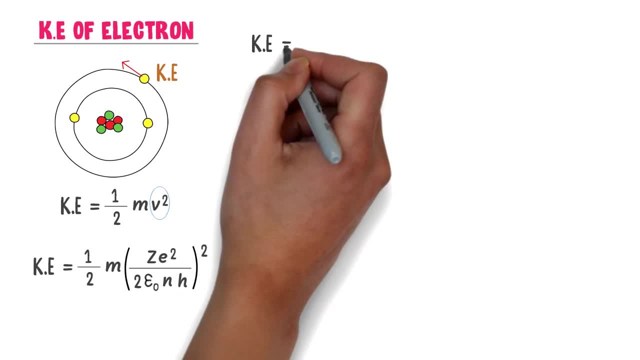 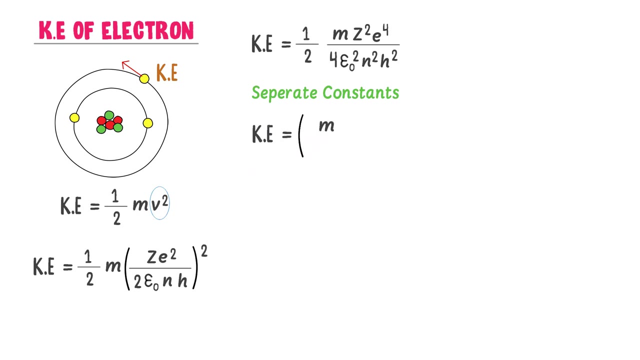 whole squared, I get: kinetic energy is equal to half mz squared, e4 upon 4 epsilon squared, n squared, and h squared. Now I separate the constant terms. I get kinetic energy is equal to m, e4 upon, at epsilon squared, h squared into z squared upon n squared, After putting the values of constant in. 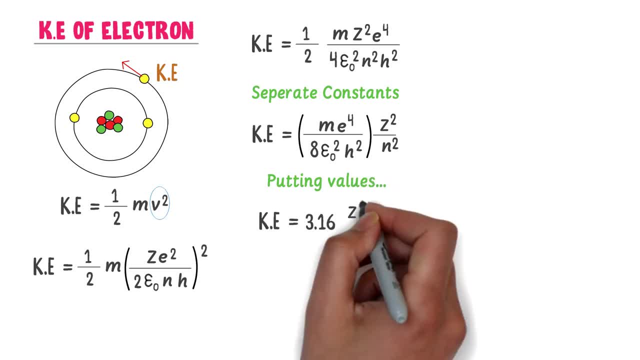 this equation, I get: kinetic energy is equal to half mz squared e4 upon 4 epsilon squared h squared, I get: kinetic energy is equal to 3.16 z squared upon n squared electron volt. So this is the kinetic energy of electron and Bohr's orbit. Here let me teach you one numerical question. 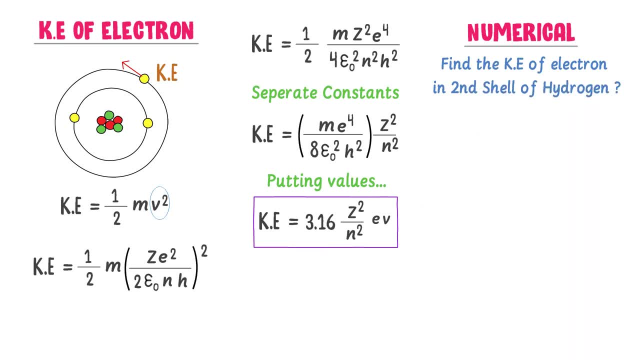 Find the kinetic energy of electron and second shell of hydrogen. Well, we know that when n is equal to 2 at a second shell, the atomic number of hydrogen z is equal to 1.. So kinetic energy is equal to 3.16 into 1 squared upon 2 squared, We get kinetic. 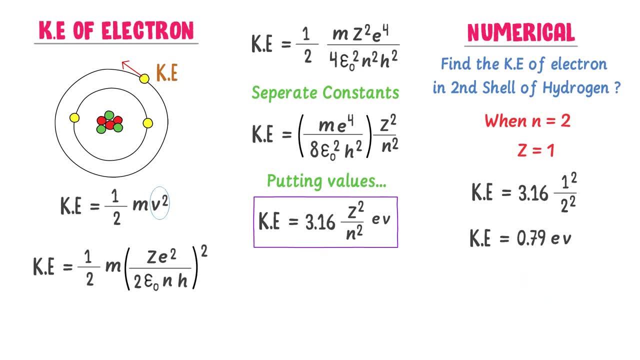 energy is equal to tron volt. Remember that sometime you are asked to find the kinetic energy of electron and kilojoule per mole. So one electron volt is equal to 96.4 kilojoule per mole. This is the energy of electron and second shell of hydrogen. 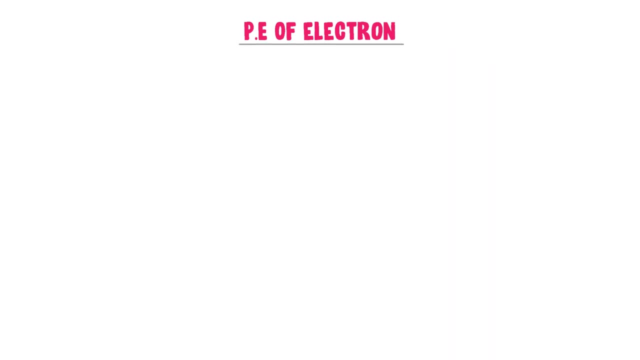 Now let me derive the potential energy of electron and Bohr's orbit. Well, let consider an electron at infinity. Let its potential energy is 16 joule. Now I bring this electron from infinity to a point where it experiences the attractive force of nucleus. So its potential. 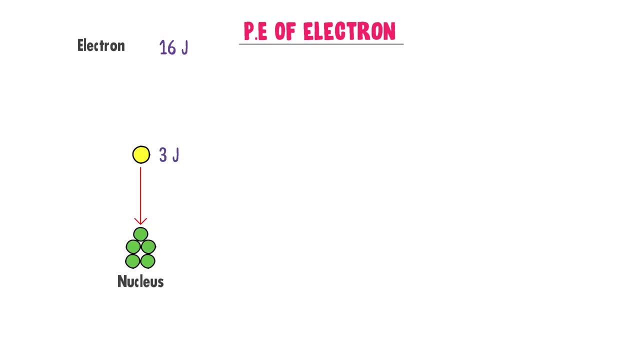 energy decreases to 3 joule. Now the potential energy of electron at this point is pe is equal to r. Remember that this negative sign shows that potential energy of electron decreases when it is brought from infinity. This f is the electrostatic force between electron and nucleus. 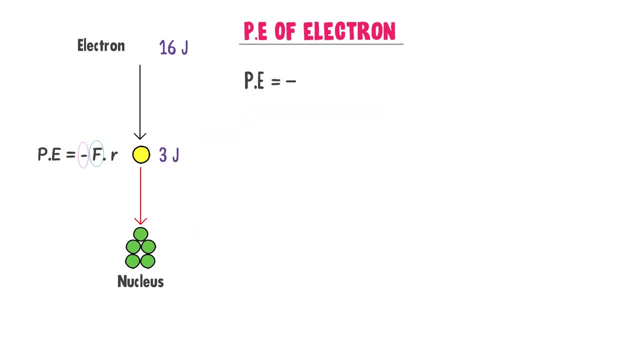 So I write: potential energy is equal to negative 1 upon 4 pi epsilon into ze, squared upon r, squared into r, This r and square is cancelled. I get: potential energy is equal to negative 1 upon 4 pi epsilon into ze, squared into 1 upon r. Let. this is equation. 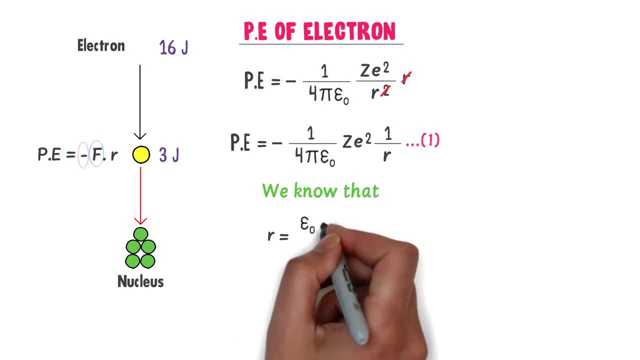 number one. We know that r is equal to epsilon n square h square upon ze squared m pi. Taking reciprocal of r, I get 1 upon. r is equal to ze square m pi upon epsilon n square h square Let. this is equation number two. 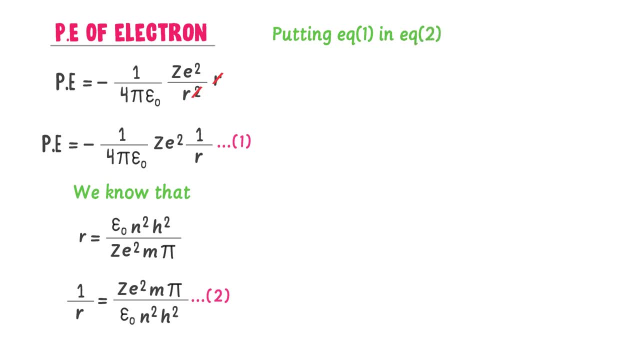 Number 2, now putting the value of radius in this equation I get potential energy is equal to negative. 1 upon 4 pi. epsilon n to z e square m. pi upon epsilon n. square h square. This pi and this pi are cancelled. 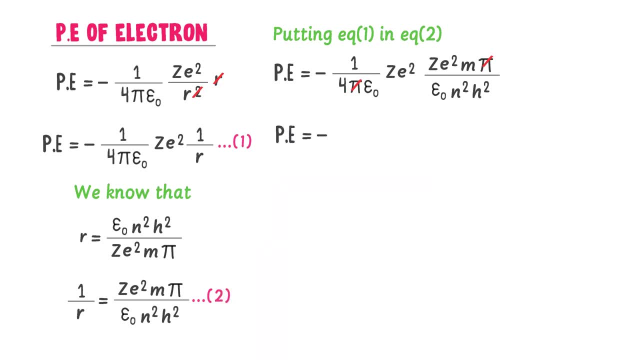 I get: potential energy is equal to negative, z squared e 4 m upon 4 epsilon square, n square and h square. Now I separate the constant terms: Potential energy is equal to negative e 4 m upon 4 epsilon, h squared, n to z squared. 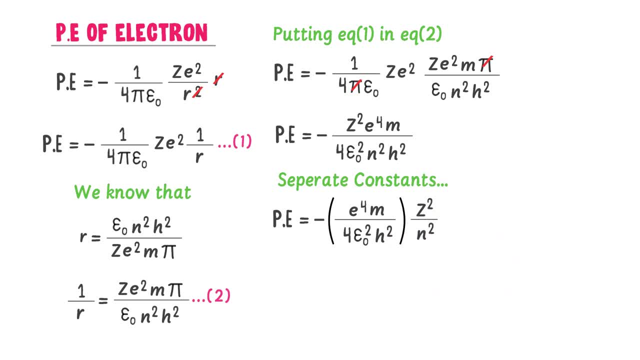 upon n squared. After putting the values of constant I get potential energy is equal to negative 27.2 n to z squared upon n squared electron volt. So this is the potential energy of electron And Bohr's orbit. Here let me teach you one numerical 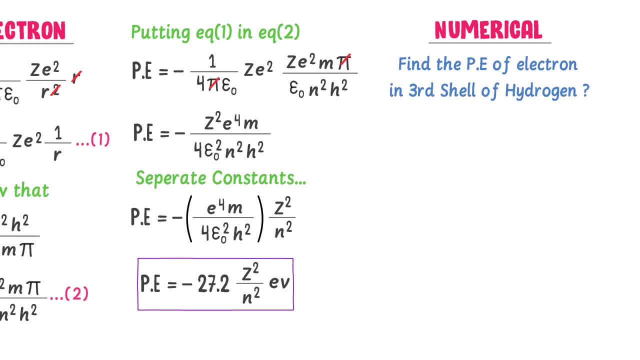 Find the potential energy of electron and third shell of hydrogen. Well, when n is equal to 3, it is third shell. The atomic number of hydrogen z is equal to 1.. So I get negative 27.2 n to 1 squared upon 3 squared electron volt, or I get potential. 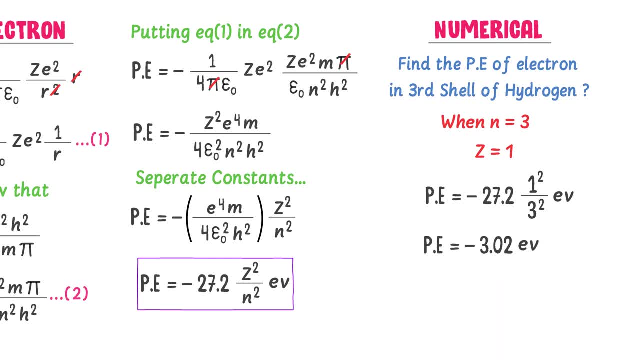 energy is equal to negative 3.2.. So this is the potential energy of electron and Bohr's orbit. We have already learned that one electron volt is equal to 96.4 kilojoule per mole. So we can also write that potential energy is equal to negative 221.4 kilojoule per mole. 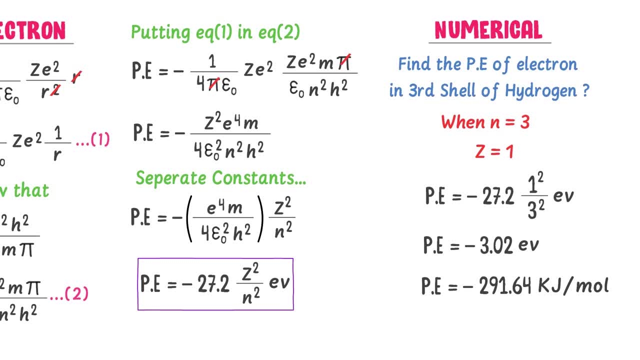 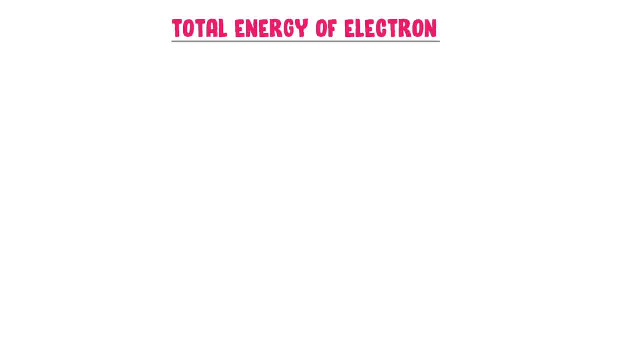 Thus, this is the potential energy of electron and third shell of hydrogen. Finally, let me derive the total energy of electron and Bohr's orbit. We know that The total energy of electron is equal to potential energy plus kinetic energy. We have already derived the values of potential energy and kinetic energy. 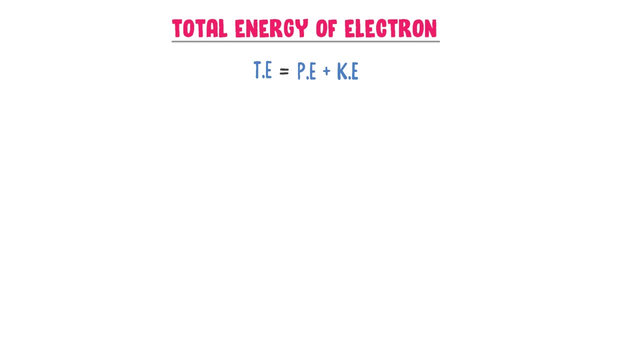 So I put the values of potential energy and kinetic energy in it I get: total energy is equal to negative z squared e4m upon 4 epsilon squared. h squared n squared plus z squared e4m upon at epsilon squared. Now I take the common parts by factorizing this equation. 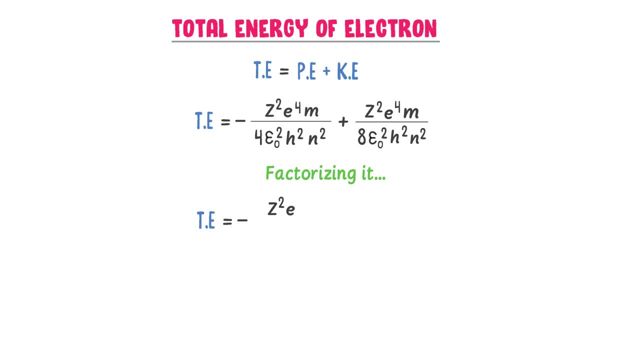 So I get that Total energy is equal to negative z squared e4m upon 4 epsilon squared h, squared n, squared n, to 1 minus 1 upon 2.. I get total energy is equal to negative z squared e4m upon 4 epsilon squared h squared. 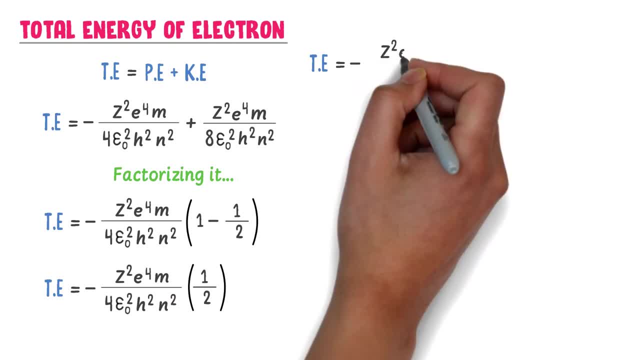 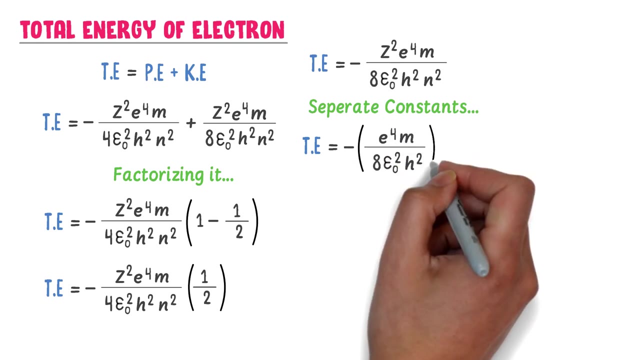 n squared, Total energy is equal to negative z squared e4m upon at epsilon squared- h squared n squared. I separate the constant terms: total energy is equal to negative e4m upon at epsilon h squared and to z squared upon n squared. After putting the values of constant I get: total energy is equal to negative 13.6 z squared. 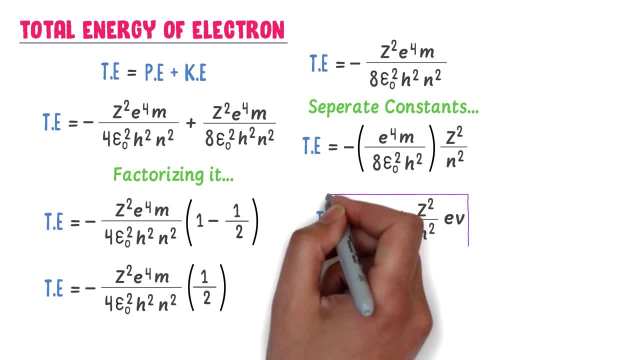 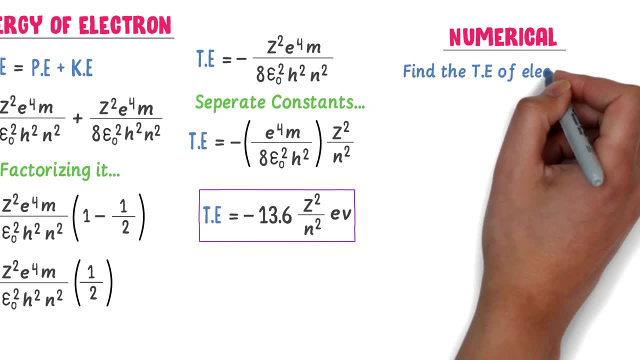 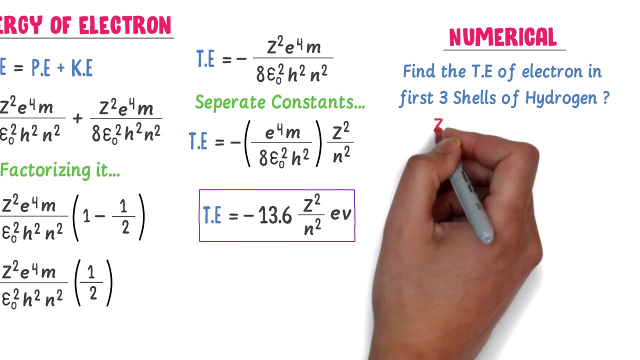 upon n squared electron volt. So this is the total energy of electron and Bohr's orbit. Finally, let me teach you one numerical question. Find the total energy of electron, and first three shell of hydrogen atom. Well, the atomic number of hydrogen z is equal to 1..